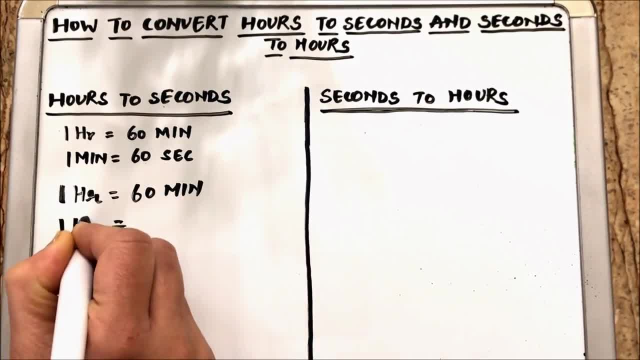 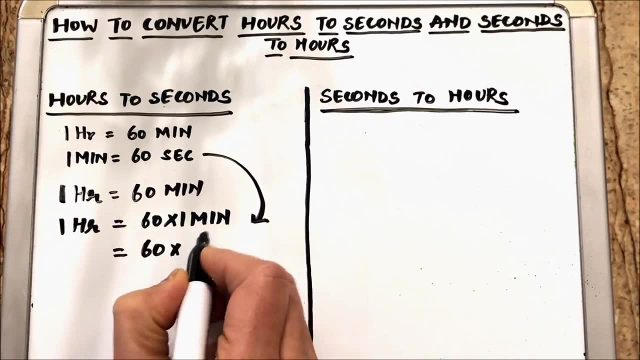 but 60 times one minute. we can write it like this: So we all know that one minute is 60 second. so we'll find hours in terms of seconds. so we'll write one minute as 60 seconds. so one hour is 60 times 60 is 3600 second. so this is now. 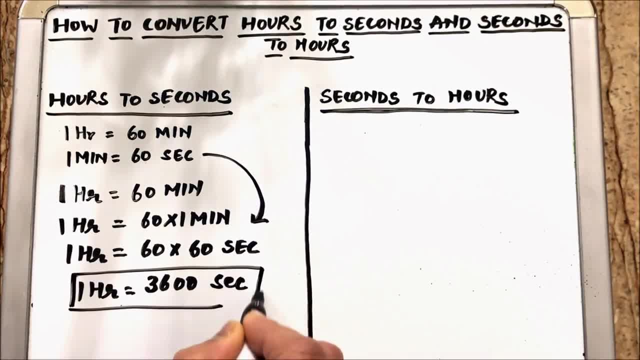 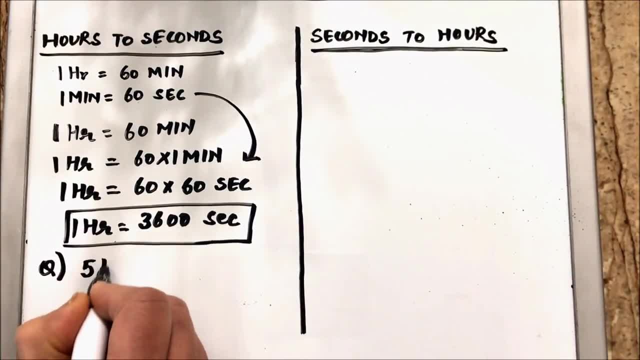 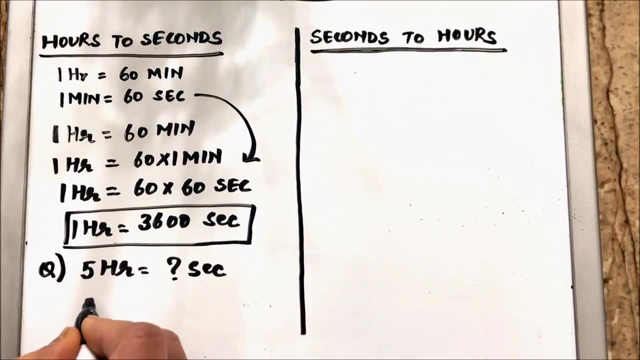 we know this is the relation. we know that between hour and seconds, this is the relation. so if we have a question to convert 5 hours is how many seconds? or to convert hours to seconds. so we all know that 5 hour we can write 5 hours as. 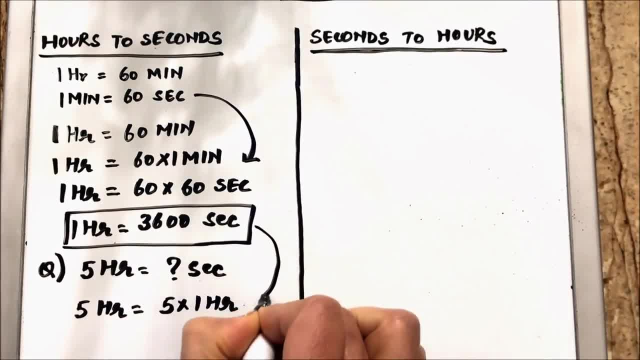 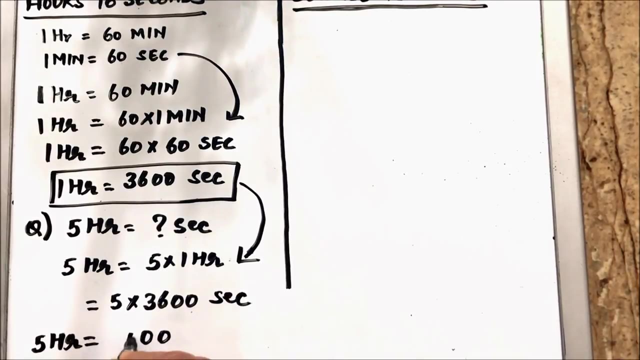 5 times 1 hour, and in place of 1 hour we will write it as in terms of seconds, which is 5 times three, six, zero, zero seconds. so five hour will be equal to zero, zero, zero. this is three, five. three is a 15, 18,000 seconds. so in this way we can convert any hours. 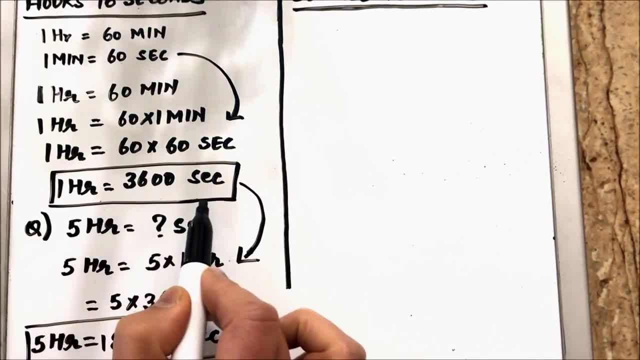 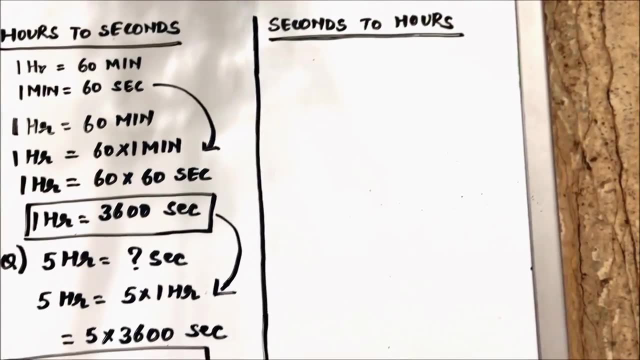 to second. we should first know the relation between hour and seconds. basic relation is this: one hour is 3600 seconds and then we can calculate from there. we can put the value of hours in terms of second and we can find the number of seconds in that many hours now. now we'll go to seconds, to our conversion. 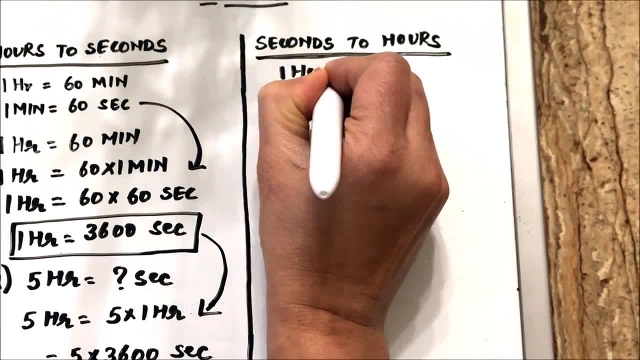 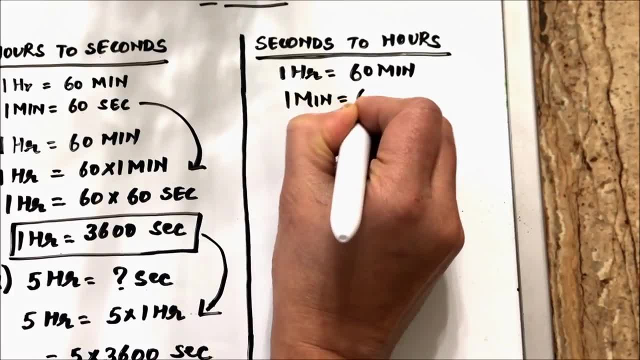 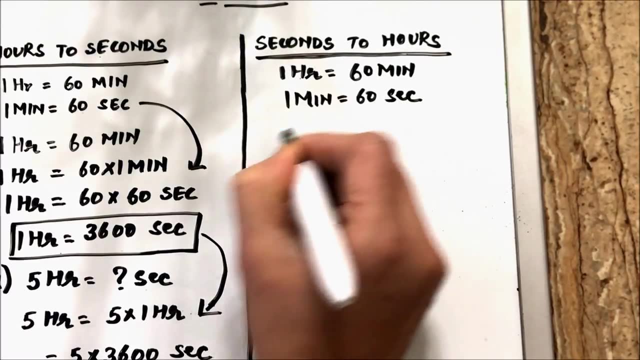 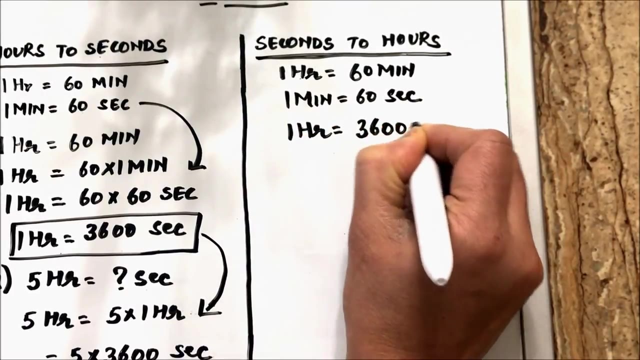 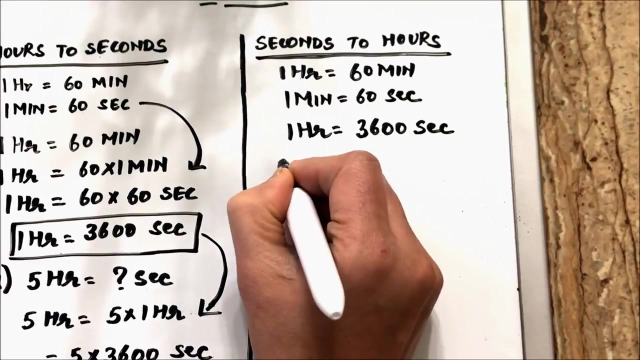 here also we will use the basic relations: one hour is 60 minute and one minute is 60 seconds. so what we need to know is from here we already know that one hour is 3600 seconds. we find from here so this relation. we can write it as one hour is.